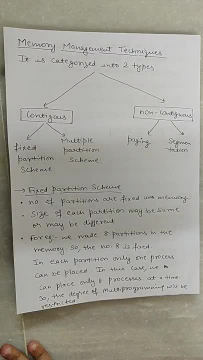 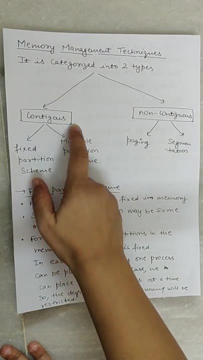 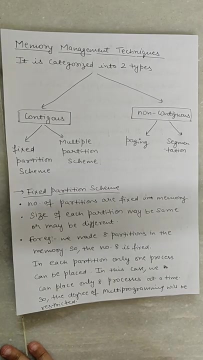 Hello everyone, welcome to operating system tutorial. In the previous lecture I have discussed memory management techniques and I have discussed the first technique, that is, contiguous memory allocation, and I have also discussed the fixed partition scheme and multiple partition scheme. In this lecture I will discuss about the issues we face in 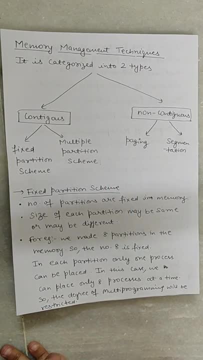 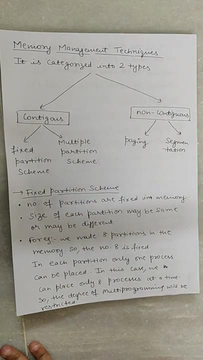 contiguous memory allocation. So if you haven't watched my previous video, please go and watch the fixed partition scheme and multiple partition scheme. So let's discuss the issues we face in this contiguous memory allocation. So we face two issues, actually two issues. 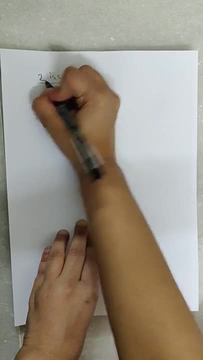 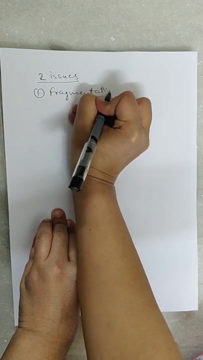 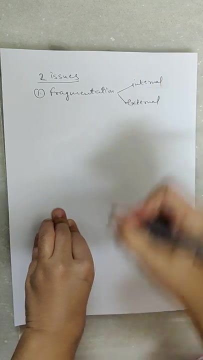 in contiguous memory allocation. First issue is fragmentation, which I have already discussed. fragmentation, Two types of fragmentation: internal fragmentation and external fragmentation. In internal fragmentation it happens in fixed partition scheme and external fragmentation happens in various types of fragmentation. So in internal fragmentation it happens. 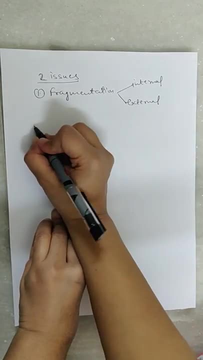 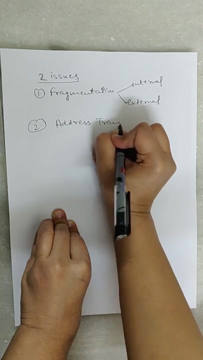 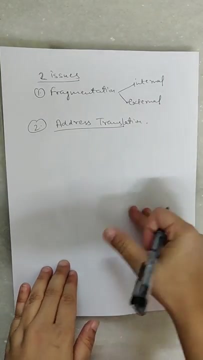 in variable partition scheme. We have discussed this. So the next issue is. second issue is address translation. I will discuss this issue in this tutorial. So before discussing this, let's take an example: What happens here? Here is our CPU. This is our CPU Here. 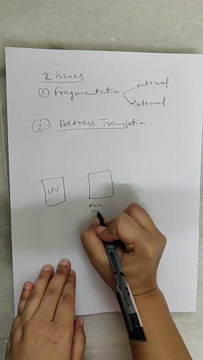 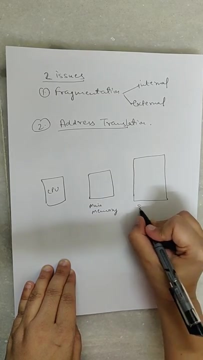 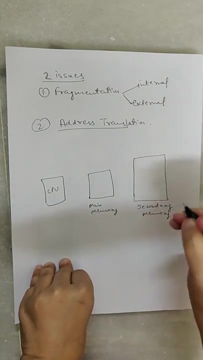 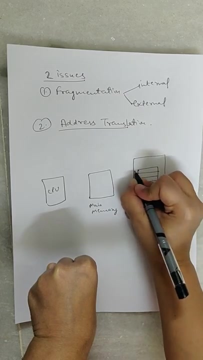 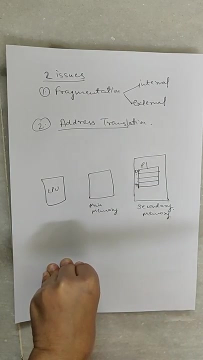 is main memory. Here is big secondary memory. Okay, Secondary memory, Okay. So now what happens? Say suppose I have a program P1. This program P1 has 50 instructions. Okay, This is my program P1. and from 0 to 49, total 50 instructions. Okay, Now this P1 program has to be executed. So 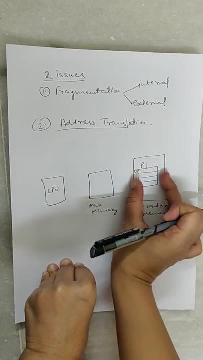 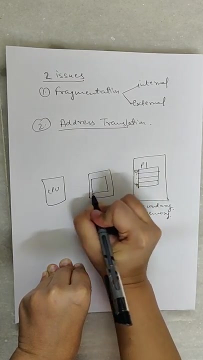 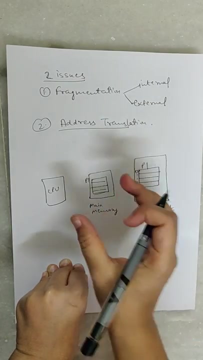 I have already told that whenever a program has to be executed, it has to reside in the main memory. Okay, So it will come exactly as it is inside this main memory. P1 has come here and since it is a contiguous memory allocation as it is, this program will be loaded in one. 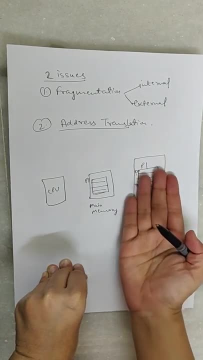 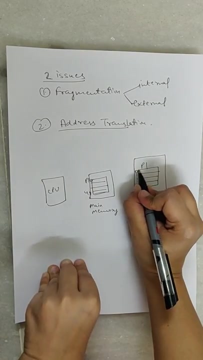 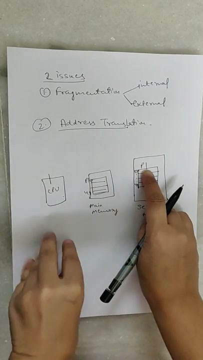 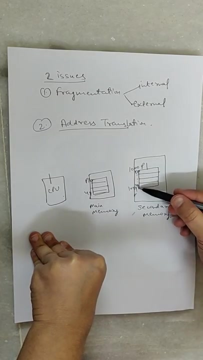 continuation. This will be loaded from secondary memory to main memory. 0 to 49 instructions. Clear. Now see Where will the CPU pick the program From here. Okay, Its address, say suppose, starts from 1000 and runs till 1049.. Okay, It starts from 1000 and runs till 1049.. And the same. 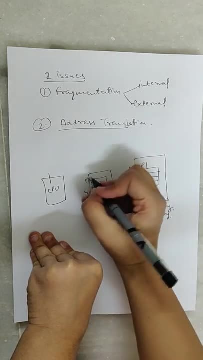 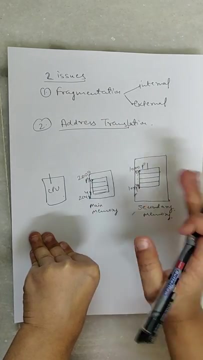 address will not be here. There will be different addresses here. Say suppose this is starting from 2000.. From 2049.. Okay, This means that its address is different in the main memory and the addresses in the secondary memory are different. Here it starts from 1000.. I have 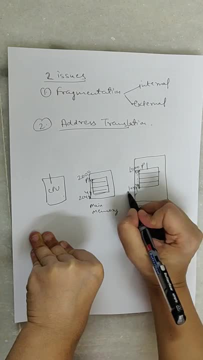 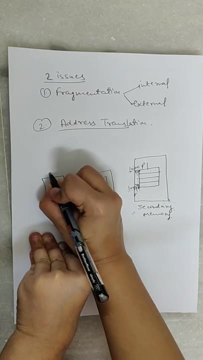 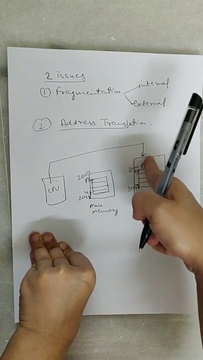 just taken an example from 1000.. Okay, Here it starts from 1000 and runs till 1049.. Here the addresses are different. Okay, Now what does the CPU do? It generates addresses for secondary memory. Okay, CPU generates addresses for secondary memory. Okay, The CPU address. 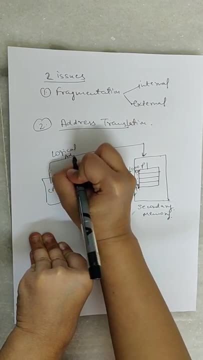 that it generates. we call it logical address. Its name is logical address, or it is also called virtual address. Okay, So it generates addresses for secondary memory. So it generates addresses for the main memory. Okay, And this logical address is the same as the address for secondary. 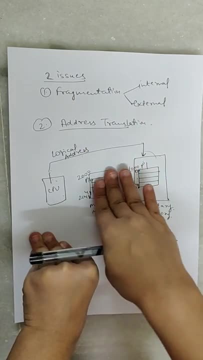 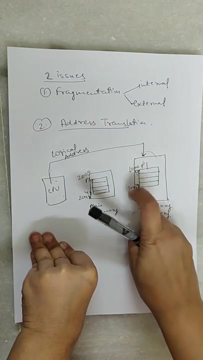 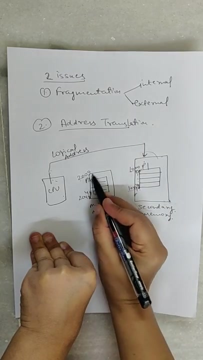 memory. Okay, CPU does not know about the main memory. Okay, CPU generates the address for secondary memory: 1000,, 2000,, 1049 and so on. Okay, So CPU does not know about the main memory. in between Clear And the addresses of the main memory, we call them physical. 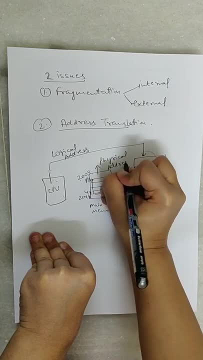 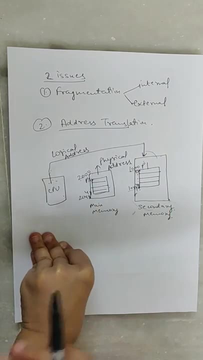 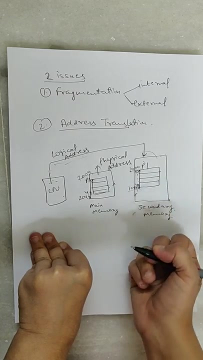 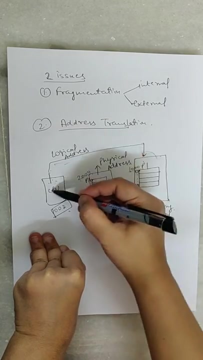 addresses Physical address: Clear, Clear. But from where does the CPU pick an instruction by instruction program to execute? From the main memory, But its address is different, so it has to execute the instruction from 1002.. Okay, So 1002 instruction is not here. The CPU is picking it from here. It is picking. 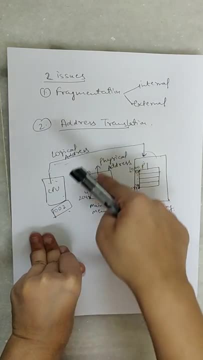 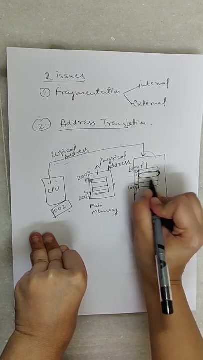 it from the main memory, But the address it has to take from here as 1002 instruction. if it starts from 1000, then 1001, 1002 will be on second number. so this 1002 instruction that we have to execute. 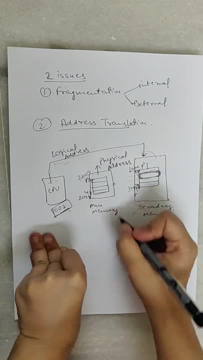 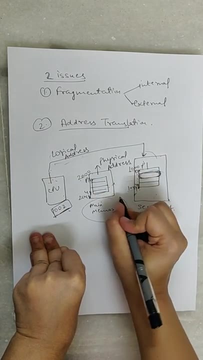 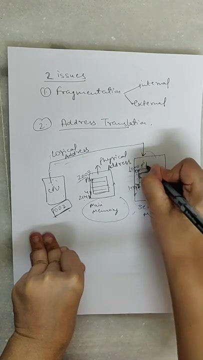 its address is given according to secondary memory. address is generated for secondary memory but pick from main memory but main memory address starts from 2000. CPU generates logical address for secondary memory but where does empty from From main memory and what is the address of main memory? It is a physical address. 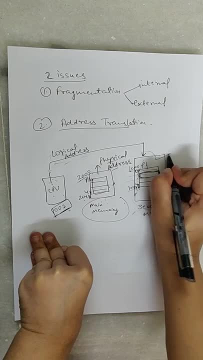 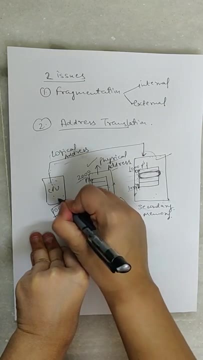 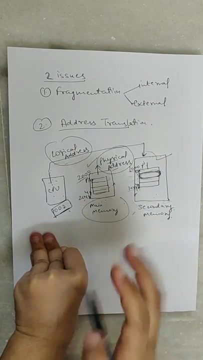 means it has a separate address of secondary memory and of main memory and CPU is generating the address for secondary memory, but where should it pick from the instruction From main memory? This address is different. this address is also different, so we have to translate logical address. 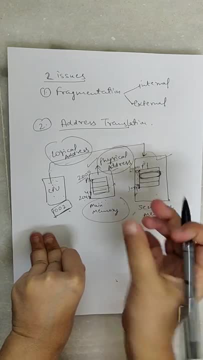 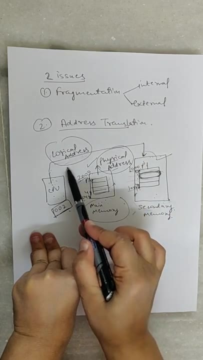 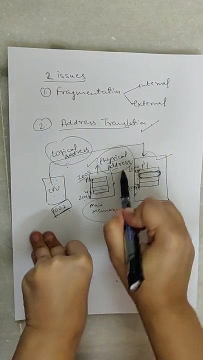 to physical address so that CPU can up the particular instruction from the main memory. So we have to translate logical address to physical address. So this is an issue which we have to resolve. We have to translate logical address to physical address. Secondary memory address is different and main memory address. 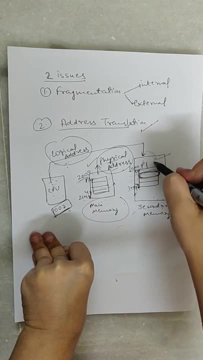 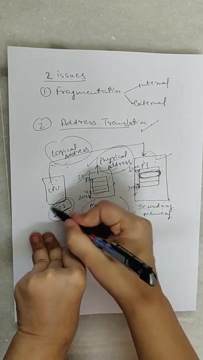 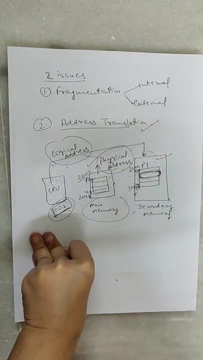 is different. CPU is generating for secondary memory. But here, where do we have to pick the instruction from? From the Main memory. But in main memory there is not 1000.2%, but 2000 is being started, So we have to do mapping logical address to physical address. Let's. 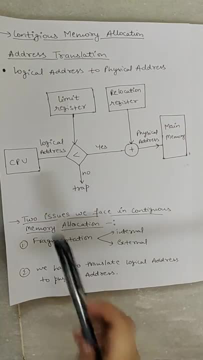 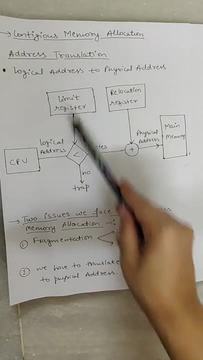 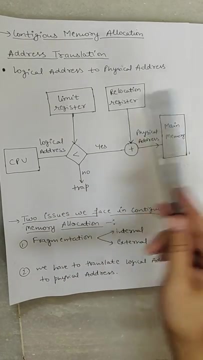 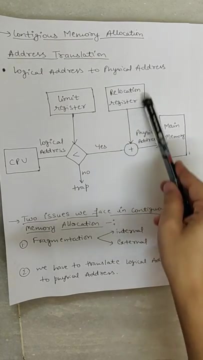 see here In this diagram, we have CPU. CPU generates logical address, So we have main memory also and main memory have physical address. CPU generates logical address for secondary memory and main memory has its own address, which is known as physical address. okay, and we also have a relocation register. this relocation register stores the base. 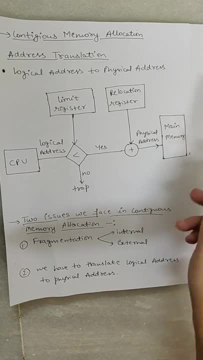 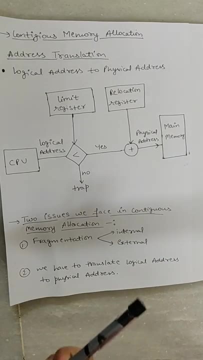 address of the particular program. okay, agar koi program hai main memory mein loaded, toh program ka jo base address hai, first address hai usko store karta hai relocation register. okay, and these are the two issues: fragmentation, internal and external fragmentation, and we have to translate. second issue is we have to 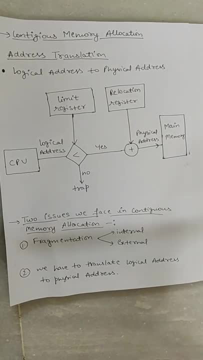 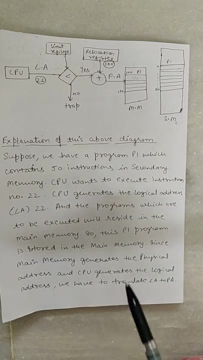 translate logical address to physical address. so just have a look of this whole diagram and take a screenshot so that I will explain it with the example also, okay, so look at this example. this is the same diagram which I have shown before also, so let's take an example. so CPU: suppose we have secondary memory, okay, 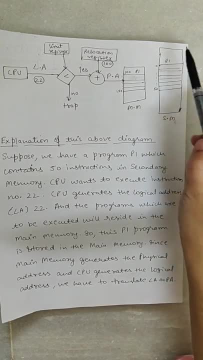 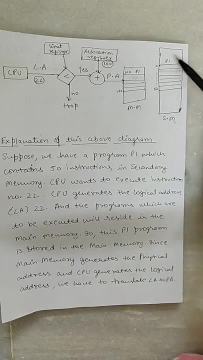 and in secondary memory I have load. I have a program P 1 which contains instruction from 0 to 50. okay, 51 instructions total in our program P1, which is starting with 0 to 50. now I have to execute this program P1. if I have to execute, then, as it is, the program will. 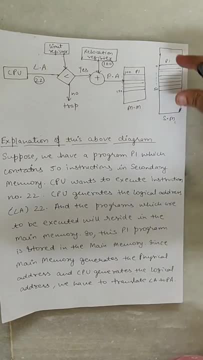 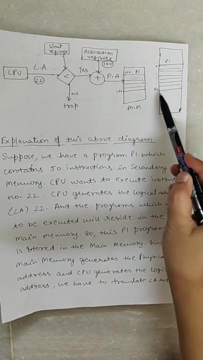 come up and will be loaded to main memory. okay, as it is, the program will come up and will be loaded to main memory. okay, main address was starting from 0. to 50 means it would first be 0 and then 1,, then 2,, then 3,, then 4. okay, so it is running like this. 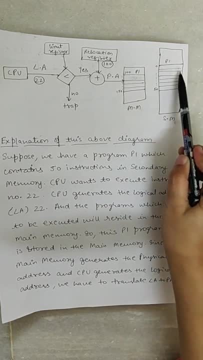 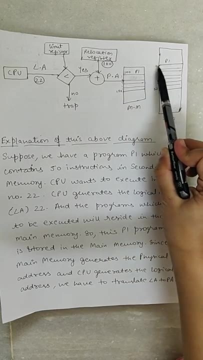 means it is running like this now here, when load is happening in main memory, then So from where it is starting? From 100 to 150.. Is it clear How it was happening here? From 0 to 50.. And what is happening here From 100 to 150. 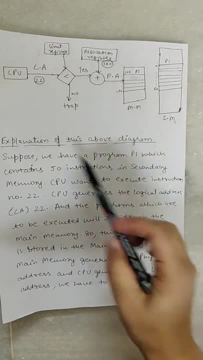 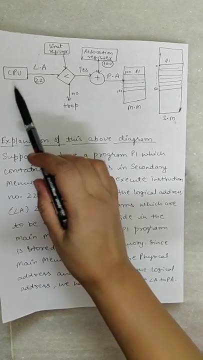 We are just taking an example Just to understand this whole process. So what is happening here From 0 to 50. And what is happening here From 100 to 150.. Now CPU has to execute program P1.. 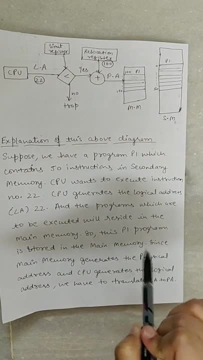 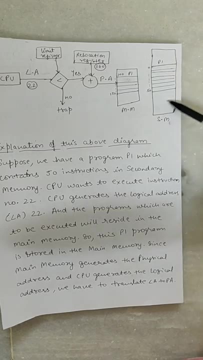 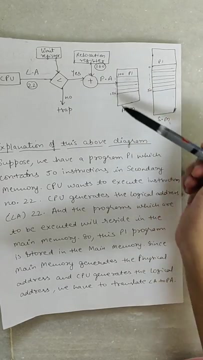 So how will it execute? Will it execute instruction by instruction? CPU is generating logical address. What does logical address mean? What is this logical address talking about? It is talking about the address of secondary memory. Okay So, But it has to pick instruction from main memory. 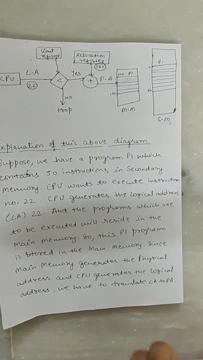 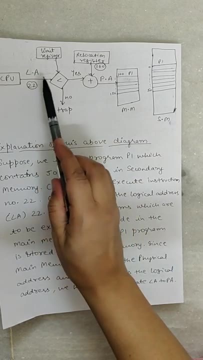 Main memory has physical address. PA stands for physical address and LA stands for logical address. Okay, So we will execute this example. now What does it say? CPU has to execute instruction no 22.. Now, according to what it has given, 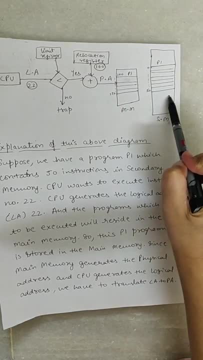 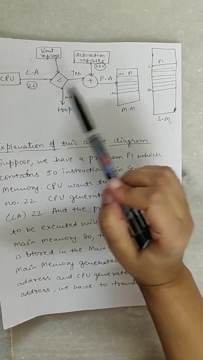 Logical address Meaning according to here. So we will keep going from 0 to 22. And it wants to execute instruction no 22. But from where will it pick? It will pick from main memory, But what did it say? 22. 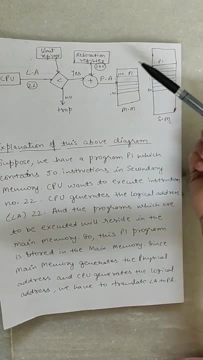 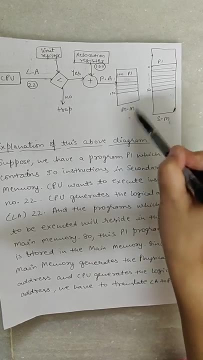 According to main memory, 22 does not reside anywhere. Why? Because it is starting from 100.. So we have to translate this 22 to physical address. So let's see how this will be translated. I will explain this part to you in a while. 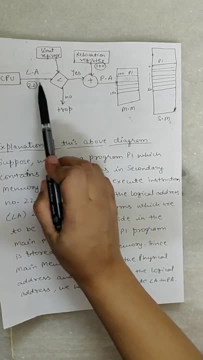 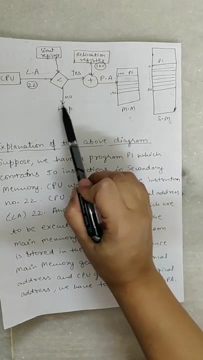 You move ahead from here. CPU has generated logical address, So it has to execute instruction no 22. Which is nothing but a logical address. Okay, We will explain this later on. Now we have come here. Now, what did I say? 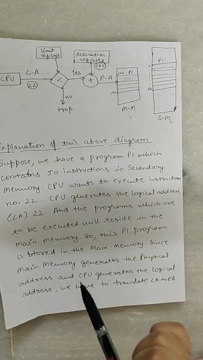 In relocation register, first instruction address is stored, Means base address is stored. Like I had told you that our main memory or our memory is like 1D array. So if we store base address in any array and we tell you that, 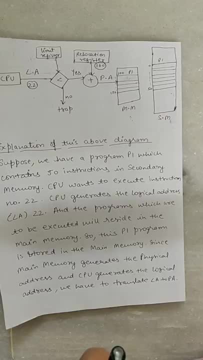 we have to go to a particular index. then you can easily find out the address of that particular index by pressing plus. So we are applying the same thing here. How are we doing it? We have to execute instruction no 22.. 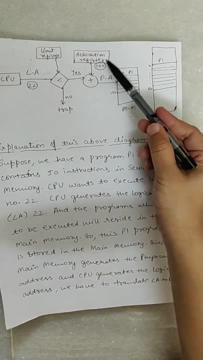 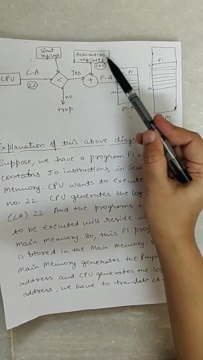 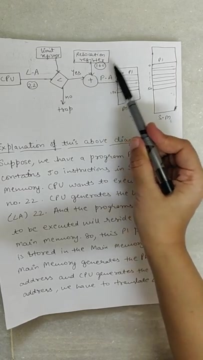 Okay, What is stored in relocation register? First instruction address means base address. Base address is nothing but 100.. So what will we do? We will add logical address with the value of relocation register. So we will add 100 plus 22. 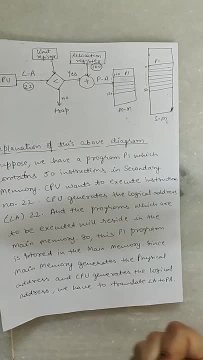 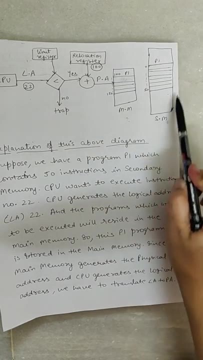 which is nothing but 122.. So we will execute 122 instruction. Okay, So this is how logical address is translated to physical address. In secondary memory the addresses were according to logical addresses, But CPU picks from main memory. 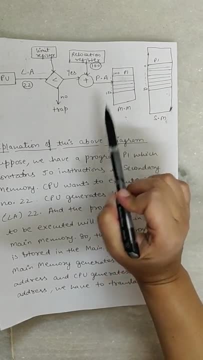 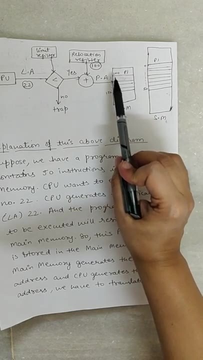 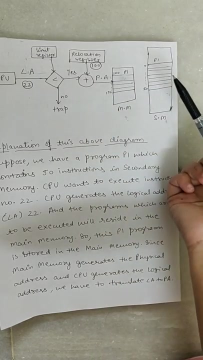 The addresses in main memory are according to physical address. We have to translate this. How will we translate? In relocation register, we will store the value of base address in logical address And we will execute the particular instruction. which will be the result. 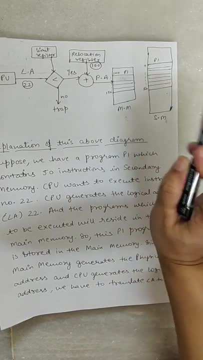 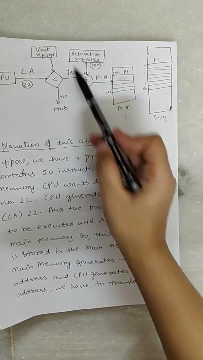 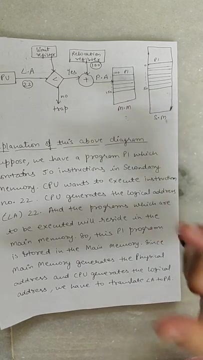 100 plus 22, we will execute the instruction no 122.. This is how we translate logical address to physical address. So now I will discuss this part. Now, what is limit register? The size of the program in the main memory. 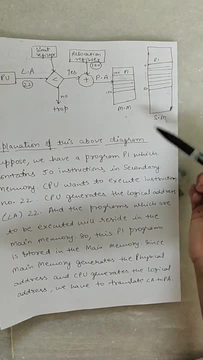 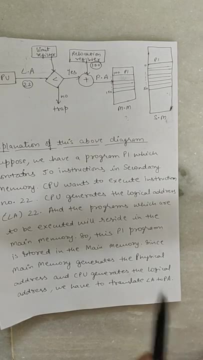 The size of the program will be same. What is the value in limit register? It is 50.. So what is the value in limit register? The size of the program? In this particular example case, what is the size? 50.. 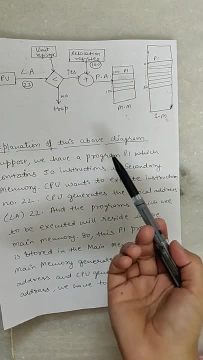 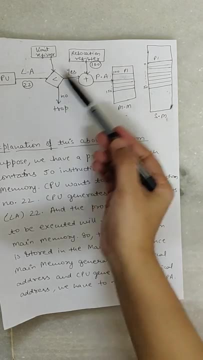 So in limit register the value will be 50. So if the value of a logical address is more than 50, let's assume it is 52. So even if it is 52, what will we do? We will not be able to. 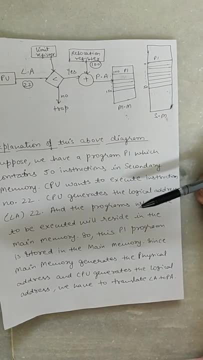 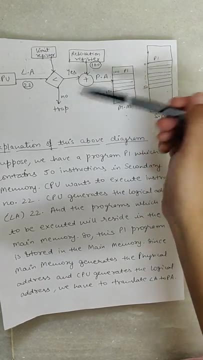 execute the program. After that, another program will start on 152.. So we are going wrong. So if something like this happens, if the value of limit register is more, then put it in the trap, Don't execute it. 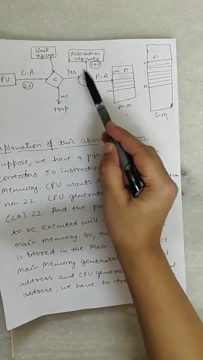 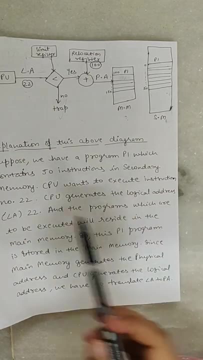 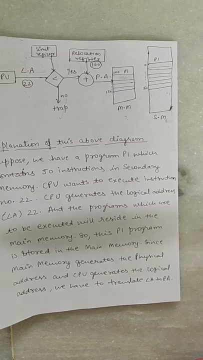 Give some error. And if it is smaller- like 22 is smaller than 50, then move forward. If yes, then move forward and translate it like this: So it will help you if you will take a screenshot. Okay, You can take the screenshot of this also. 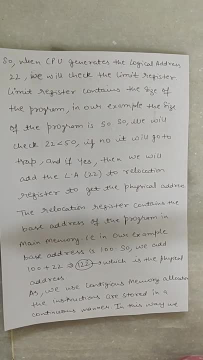 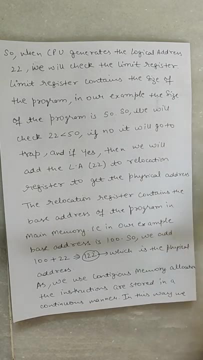 This is the next page In these notes. I have already explained this limit register. It will store this value. You have to check if 22 is less than 50. If no, it will trap And if yes then you will add the value. 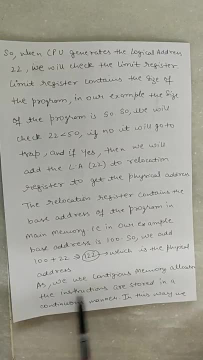 Like this, 100 plus 182, which is the physical address. So as we use the contiguous memory allocation, the instructions are stored in contiguous manner. Okay, So because of that, it will be easy for us to do this If we have base address. 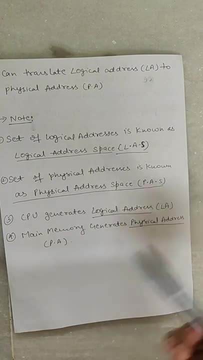 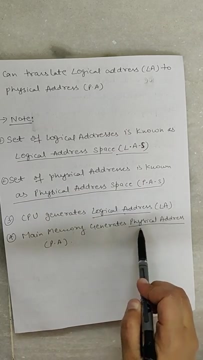 In this way we can translate LA to PA. that is, logical address to physical address. And you have to note these two things: If we say logical address, Which is logical address, It generates CPU. CPU generates logical address. Main memory generates physical address. 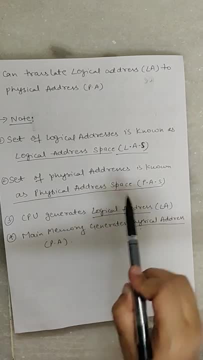 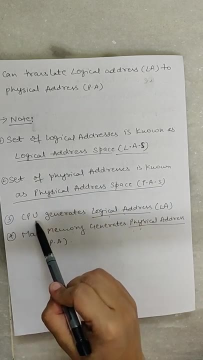 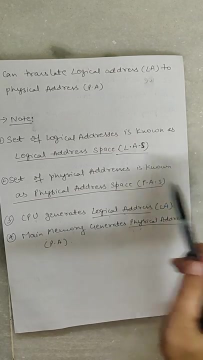 Keep this point in mind- And whose logical address is Secondary memory And whose main memory address is Physical address And who generates logical address- CPU. We can also call it logical address or virtual address, And if you make a set of